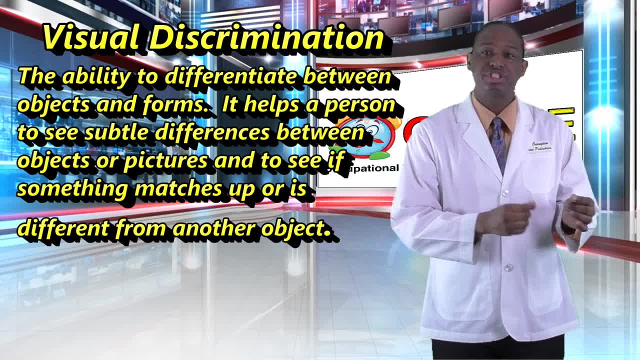 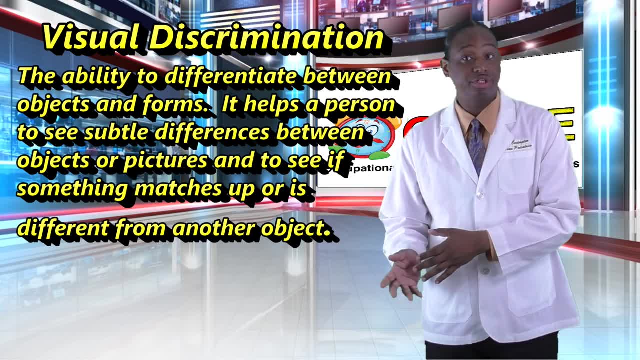 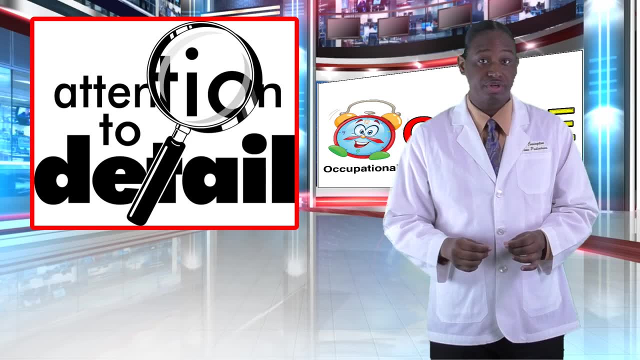 Visual discrimination helps a person to see subtle differences between objects or pictures and to see if something matches up or is different from another object. This visual perceptual skill can be described as paying attention to detail. An example would be being able to see differences between similar looking letters and words, such as 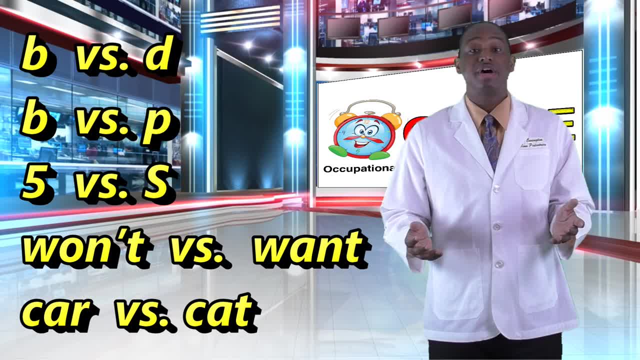 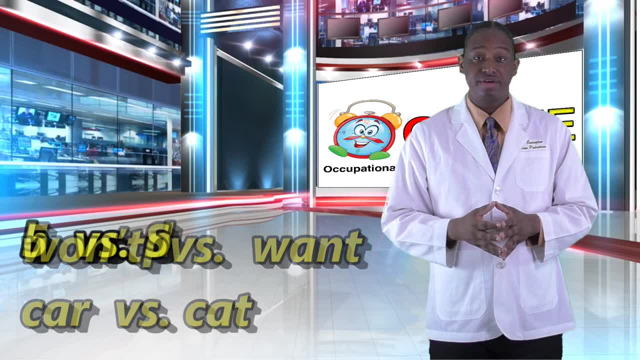 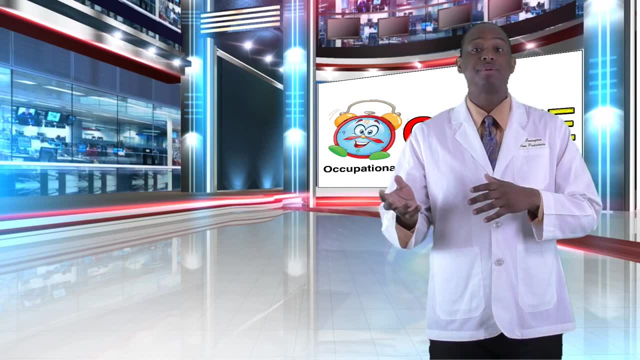 B's and D's, B's and P's, 5's and S's won't and want, or car and cat. Having deficits in visual discrimination can affect daily life as well. There could be problems in dressing, for instance, matching shoes and socks. There could be difficulties. 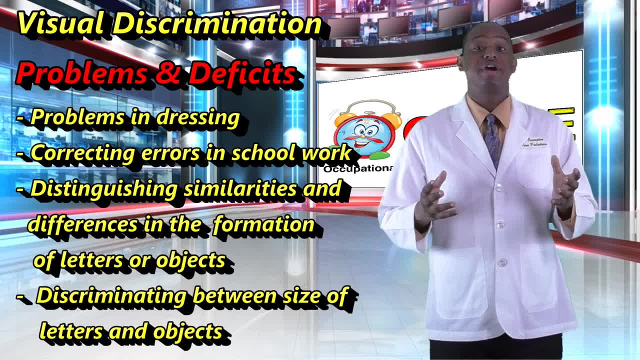 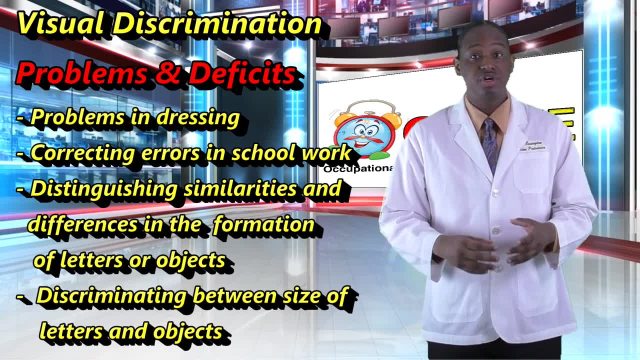 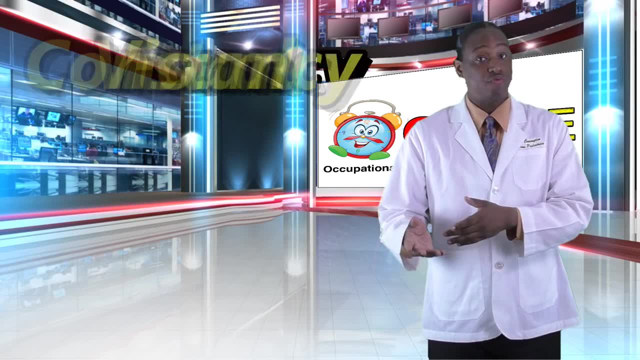 correcting errors in schoolwork. There could be problems distinguishing similarities and differences in the formation of letters And sometimes, in this case, you may see letter reversals. Next we have visual form constancy. Now, visual form constancy is the ability to recognize. 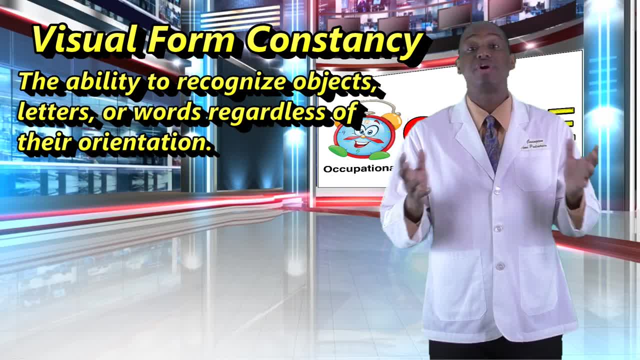 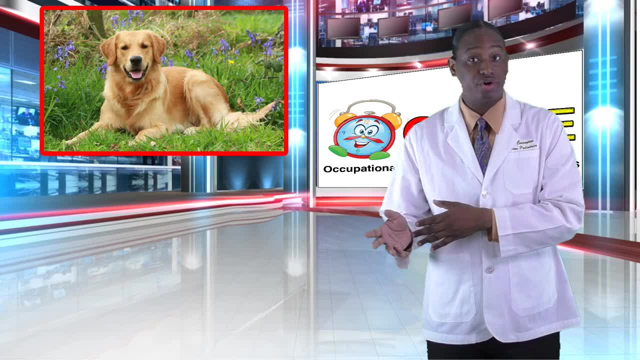 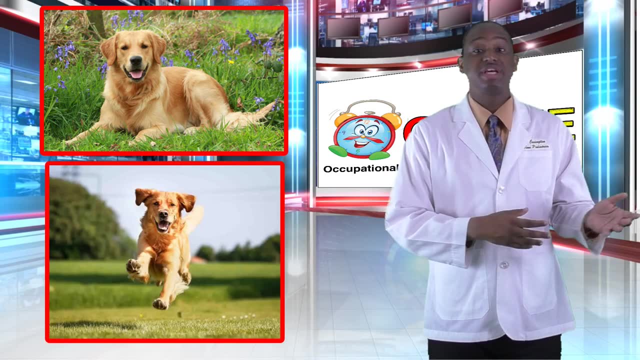 objects, letters or words, regardless of their orientation. A simple example would be that you can recognize that a dog is a dog, whether you see it in a photo, in your garden or in the park, and whether it's sitting, lying down or even running. 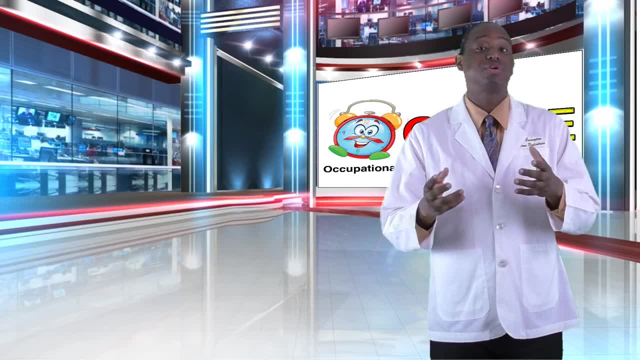 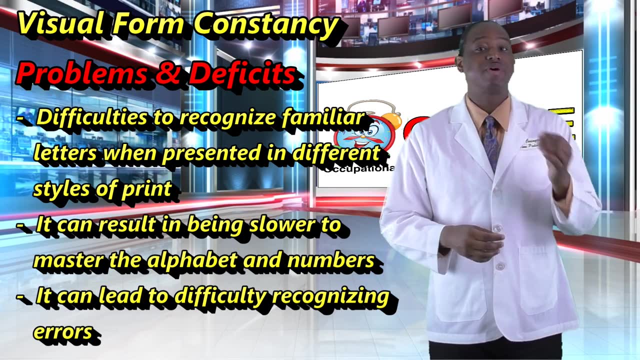 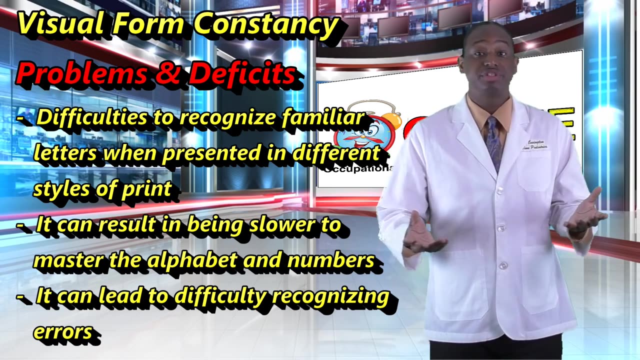 Deficits in visual form constancy can cause difficulties in a number of areas. It would make reading difficult, as a child might not recognize familiar letters when presented in different styles of print, So if the font size or the color is different they may. 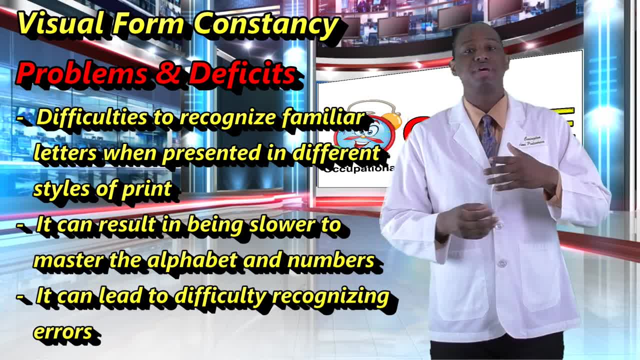 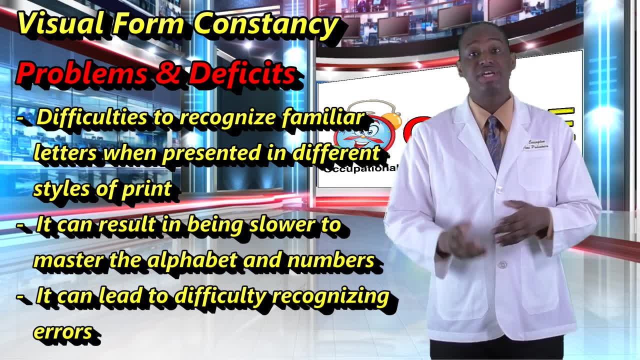 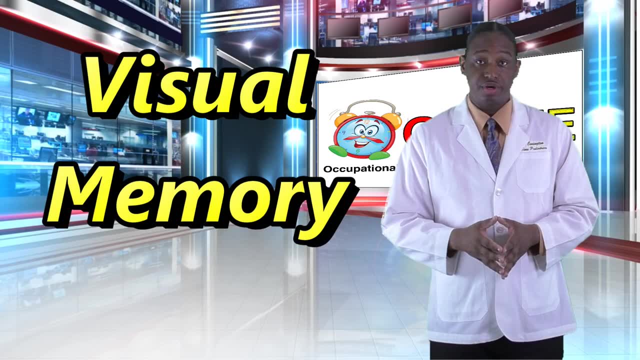 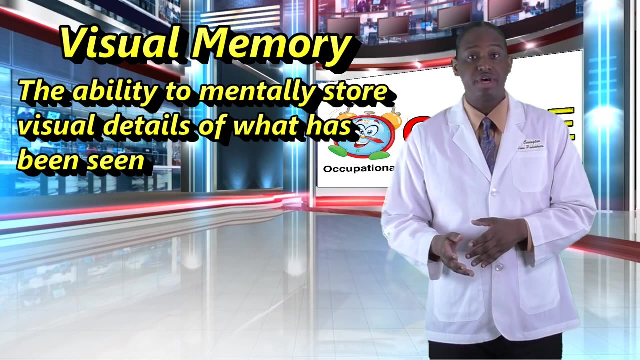 have difficulties. It can result in being slower to master the alphabet and numbers, and it can lead to difficulty recognizing errors in written work. Up next is visual memory. Visual memory is the ability to mentally store visual details of what has been seen. The ability to recall or remember the visual details of what you have seen is known as 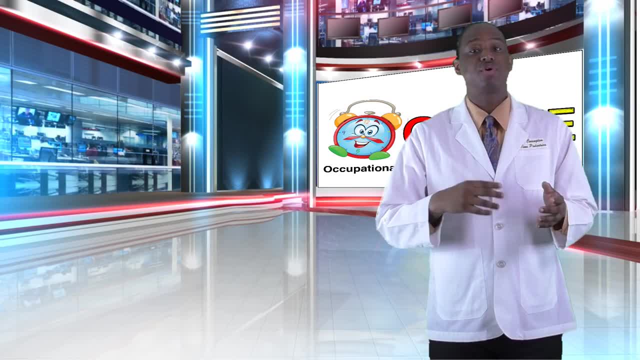 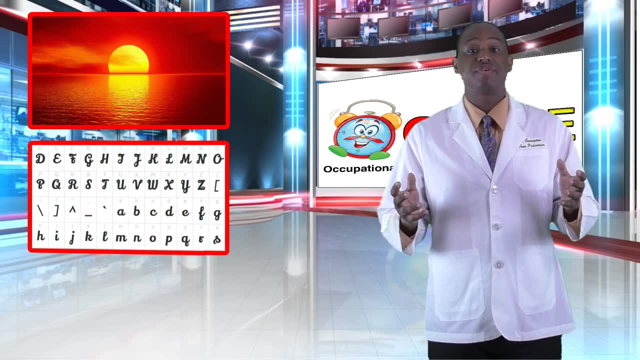 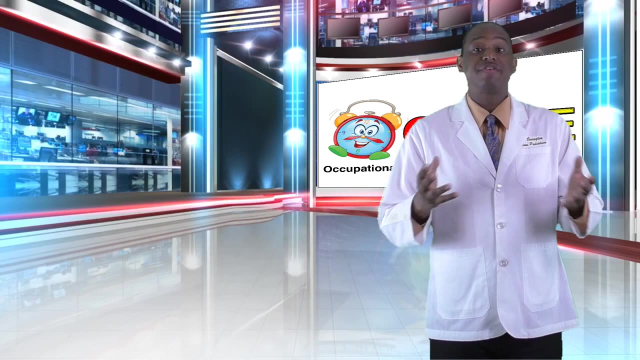 visual memory, For example, when you can recall the image of a sunset, the memory of a font type or the remembrance of a tree's appearance. these are all instances of visual memory. Now, deficits in this area may cause difficulties when recognizing numbers and letters, or 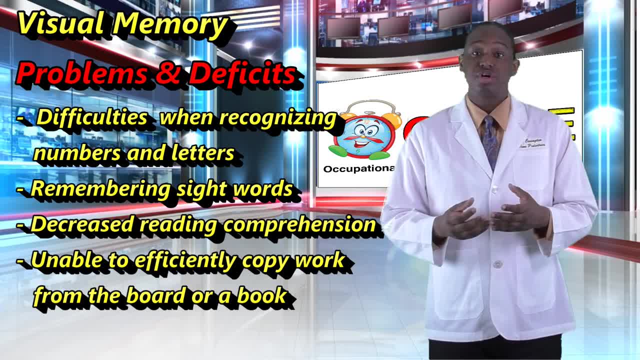 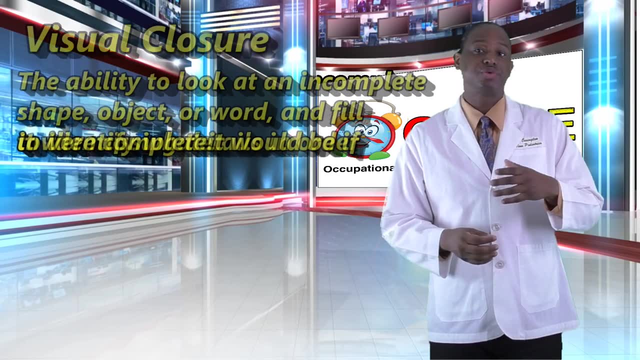 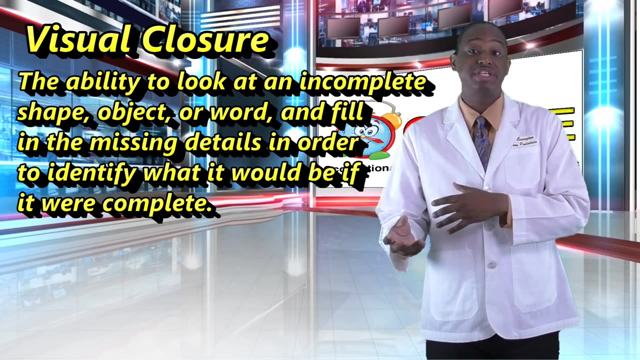 remembering sight words, one's reading comprehension or being able to efficiently copy work from the board or a book in a good time. Then there's visual closure. Visual closure refers to the ability to look at an incomplete shape, object or word and fill in the missing details in order to identify what it would. 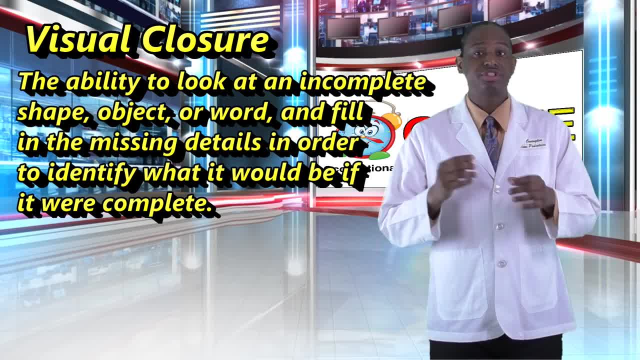 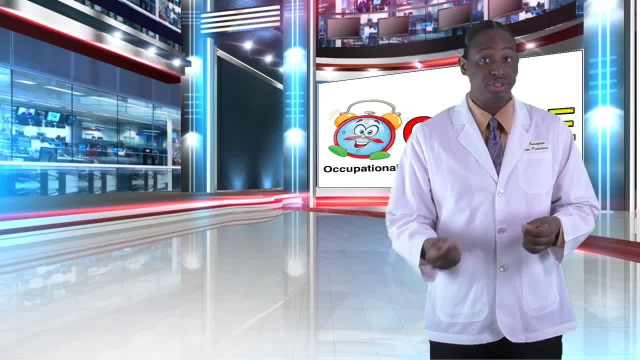 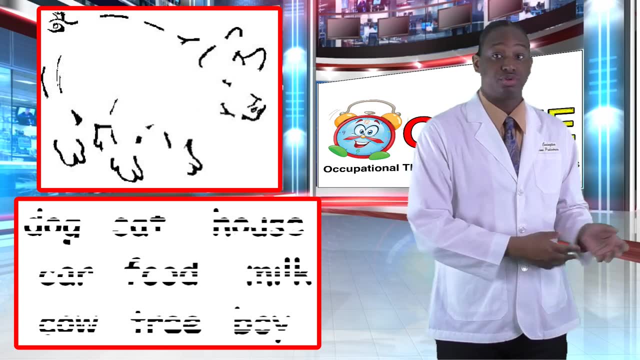 be if it were complete. It's the ability to correctly perceive something even when it's partly hidden. This skill requires abstract problem solving. This ability helps you to quickly make sense of what you see, even if it's not all visible to you, which means you do not have to see. 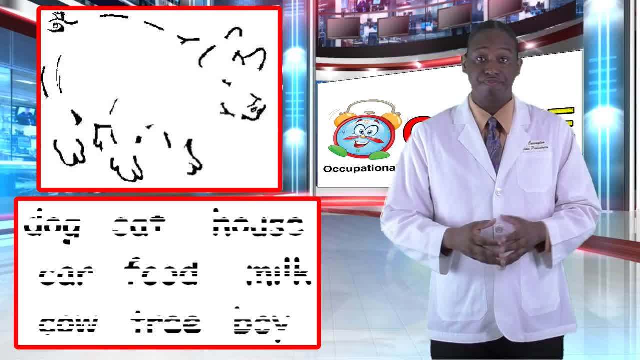 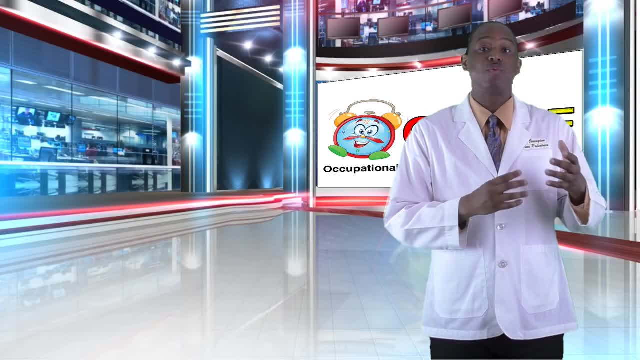 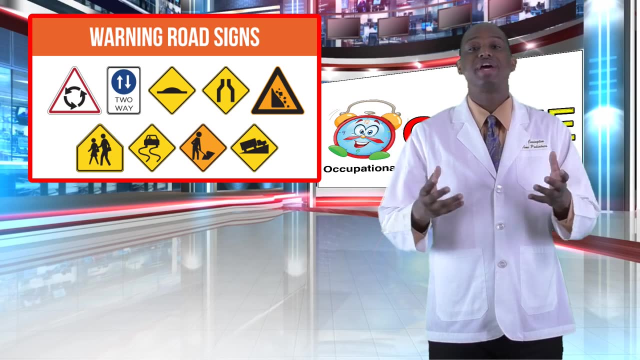 every little detail in order to recognize something. Now, an example would be: you're using visual closure skills when you can figure out what a road sign says, even if it's partially blocked by a tree, or when you're playing Wheel of Fortune on TV. also, when you can make sense of words on a smudge page, or when 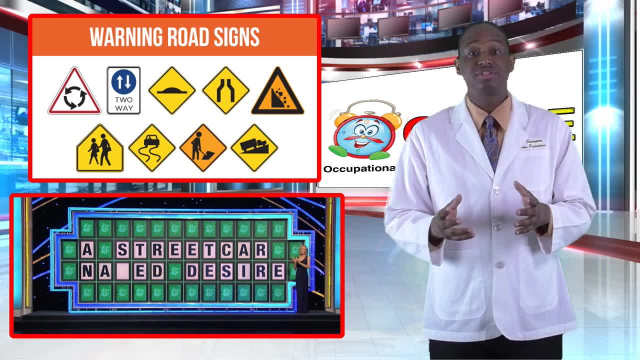 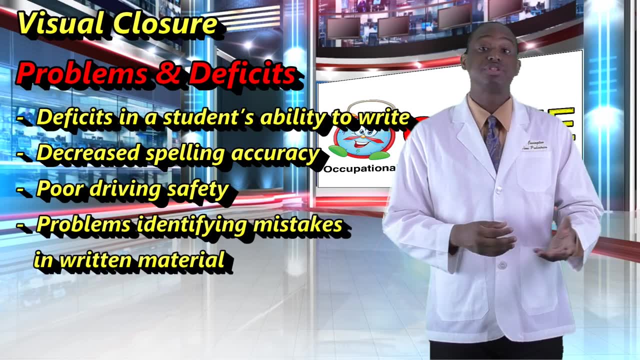 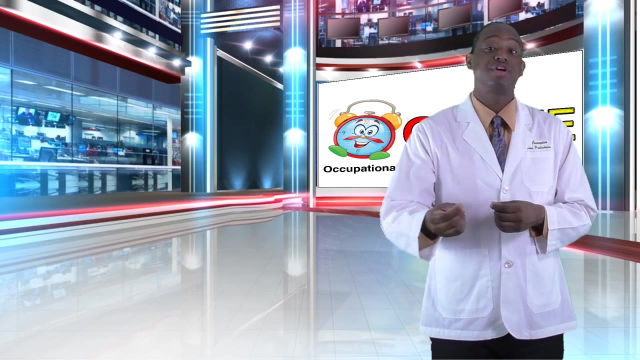 you can find a missing item when it is partly hidden. Now, poor visual closure skills can cause problems with a student's ability to write spelling words drive safely, Problem solving or identifying mistakes in written material. Lastly, there's figure ground. Now, figure ground perception is the ability to focus on one specific piece of information. 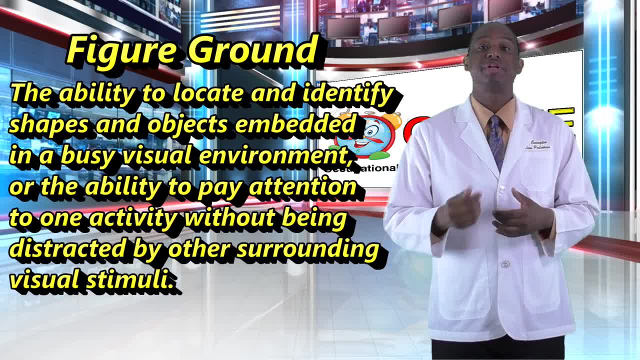 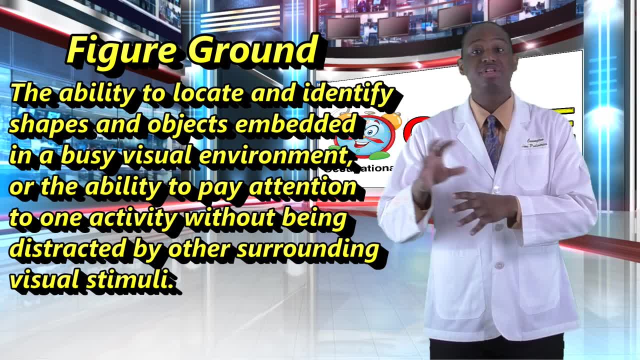 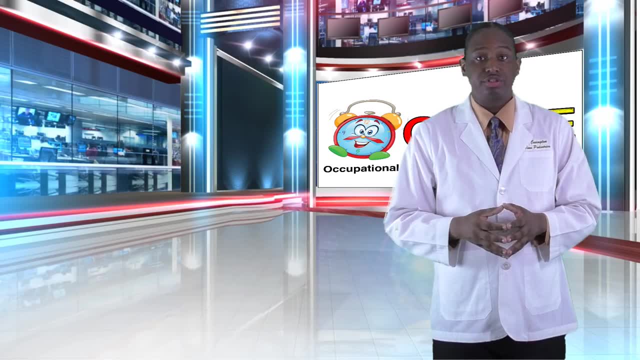 in a busy background. It refers to the ability to locate and identify shapes and objects embedded in a busy visual environment, or the ability to pay attention to one activity without being distracted by all the other surrounding visual stimuli. Some examples of visual figure ground are: finding your favorite socks in a messy drawer.